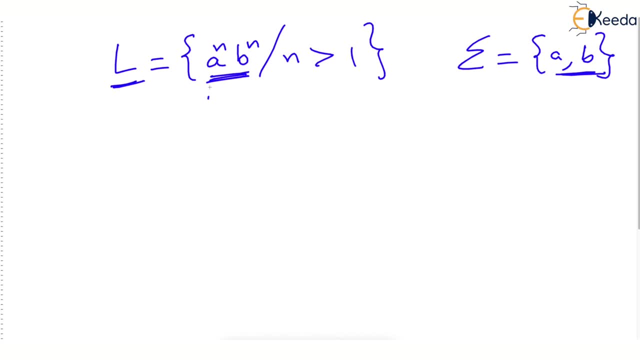 all words is a raised to n, b raised to n. So in the lead there should be some n a's and in the lag, at the end or at the tail, there should be exactly equal number of b's, But n should be greater than 1.. 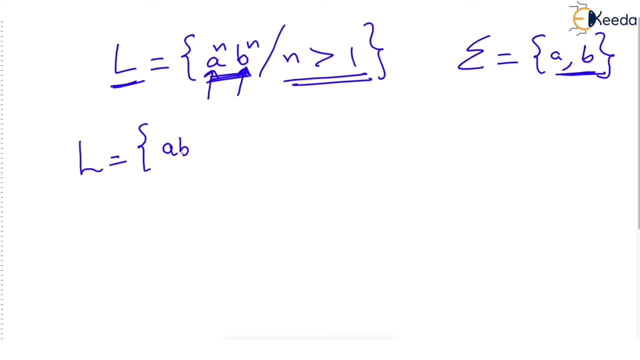 So what is this language? The smallest string in this language will be ab. This is a raised to 1, b raised to 1.. The second string will be a a b, and then a a b, and this is a infinite set of strings. 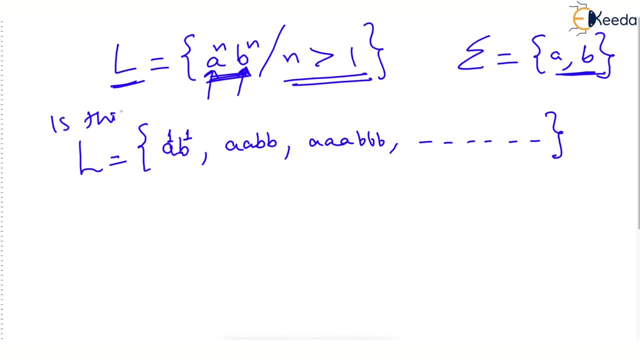 Now the problem here is that: is this language regular? Well, what do you mean by this? is that another way of asking the same question? is this language regular? Is a DFA- deterministic finite automata- or NFA, because you know both are equivalent in power. 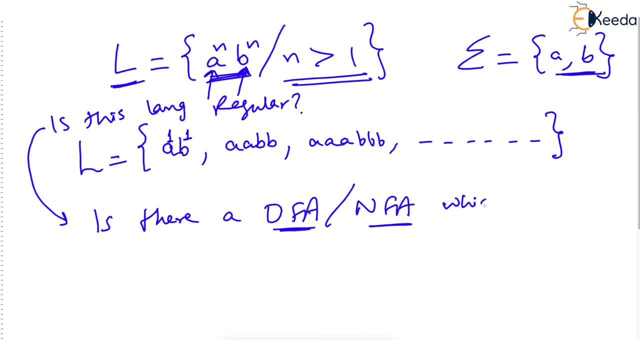 is there any DFA or NFA which can generate, generate this language? this language L is is the another way of asking. note: if there exist a DFA which can generate this language L, then we say this language is regular. I repeat, if they are exist a DFA or NFA, if we are able. 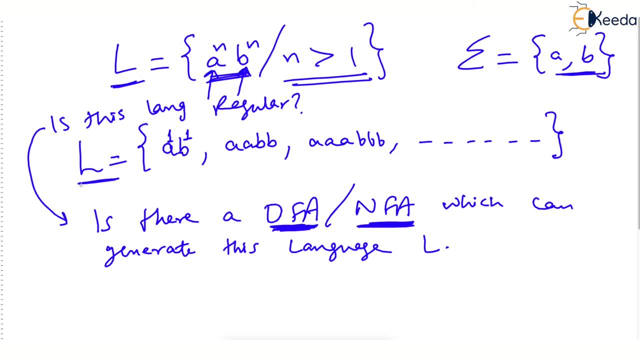 to construct a DFA or NFA which generates this language, L, which is having equal number of A's and B's. a raise to n, B raise to n is the format. then we say: this given language is regular, ok, but then the point is that they exist. 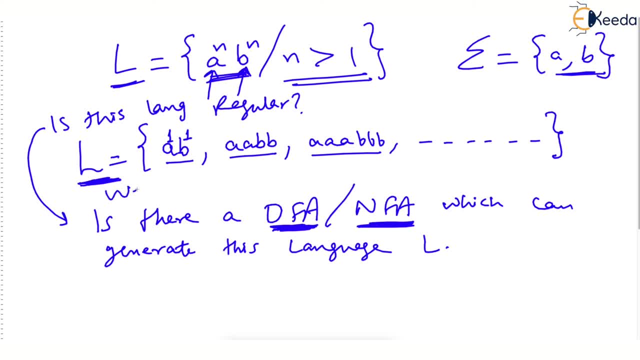 No, absolutely no DFA. I mean we cannot. we cannot create or construct DFA or NFA for the above, for the above language, For the above language. That's a big challenge actually, I mean saying that some problem is not solvable itself, needs a big courage. 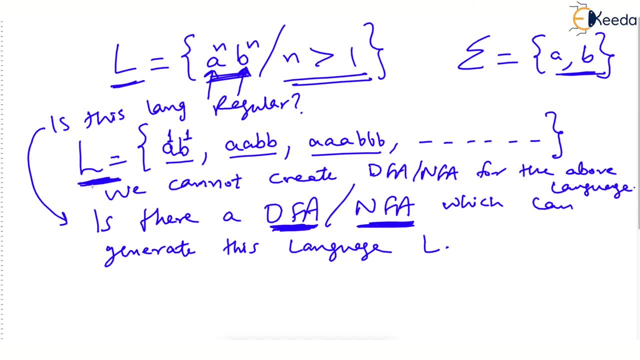 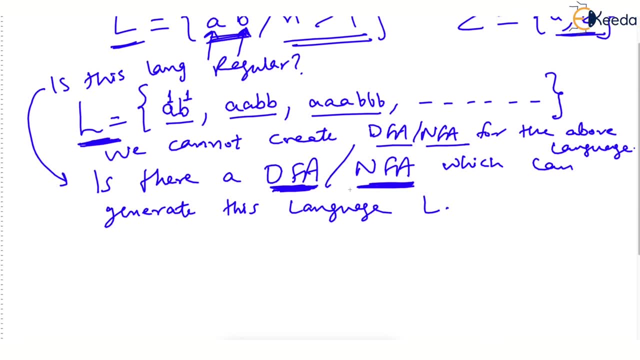 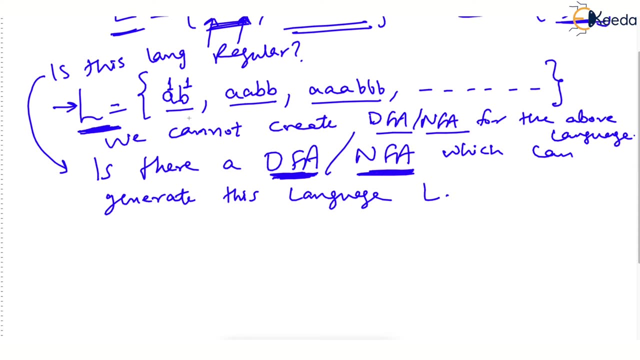 Because anybody can claim like that, that, given any language, we can say no DFA and NFA does not exist. So what I am saying is that there exists no DFA, absolutely no DFA for this language L, Then this language is not regular. 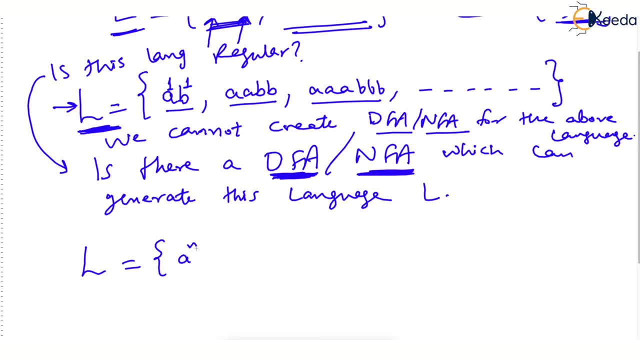 Consider another language, L, which is of the form a raised to n b, such that n is greater than 1, where sigma is a comma b. The question is: is this language regular? And the answer is yes, Because we can make a DFA. 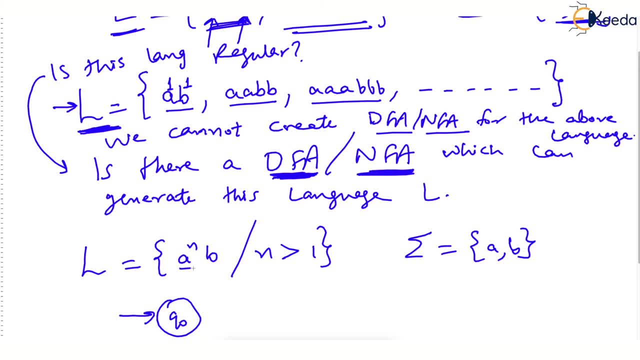 The DFA will have initial state q0. And look, initially we need some a's, but number of a's should be at least 1.. So here comes a and then we can have any number of a's- 0 or more a's. we are in q1 state. 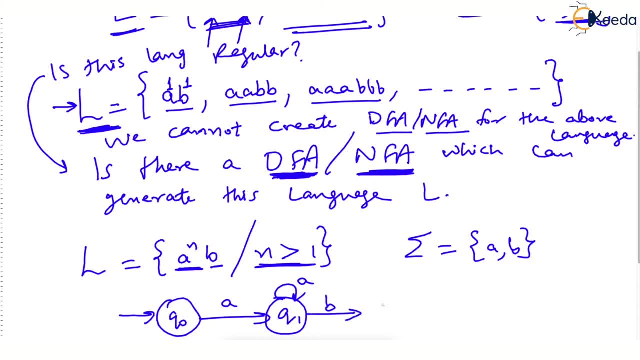 And after that the string must end with a single b. So this is the final state, And of course in the lead we should have a string of a, At least 1 a. So if we get first b, first b, then we will send it to dead state. 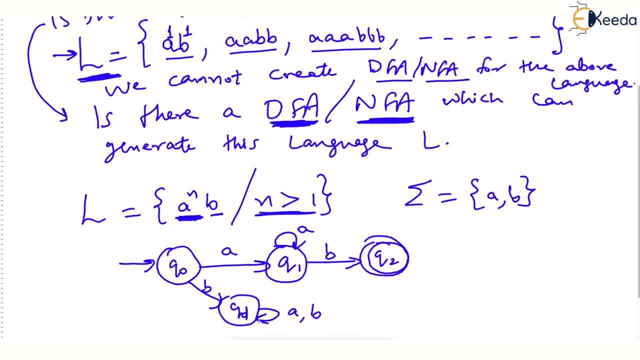 Dead state And here the machine will stay. for all other characters, The description of this DFA can be seen, because all strings of this form will be accepted by this DFA And all strings which are not of this form will be rejected. For example, what if I give a string baa to this DFA or bab? let's say: 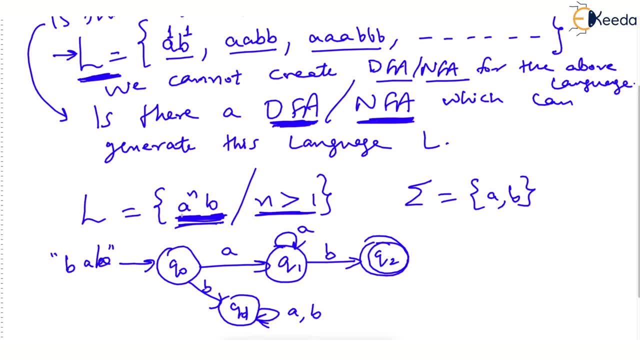 Then bab is not of this form because the string must start with a. As soon as q0,, the initial state will get the first b. it is going to send it to dead state and the machine will stay here for rest of the a's and b's and will never reach the final state. 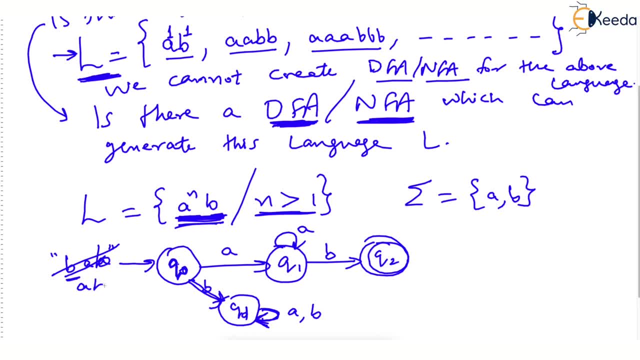 But if I give a string say as follows: ab. this is exactly. this string is exactly of this form. So after reading first a, the second b will take us to the final state. Correct. And what if? after this b, after this last b, if we get any more a's and b's, we should send it to dead state. 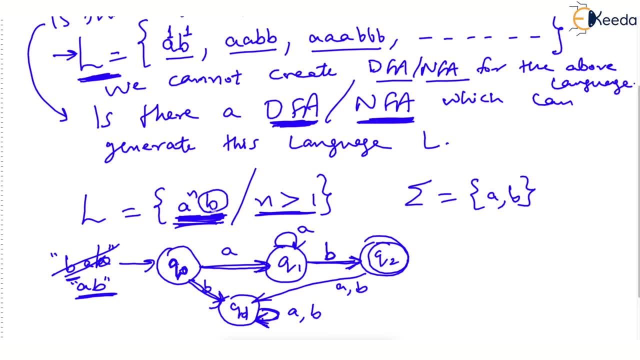 Please try to understand, because the string must end with a single b and after that single b. if we have any other letters, we don't appreciate them, isn't it? Well, the DFA is not to be taken seriously, this DFA, but what I want to prove is that we were able to construct DFA for this given language. 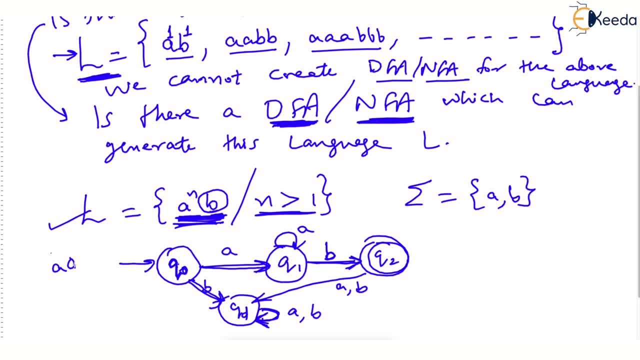 For instance, let's say I have, For a string like this, double a, b and a. this string is not the part of this language Because, you see, after this b we should have none of the characters, And this string will be definitely rejected by the given DFA. 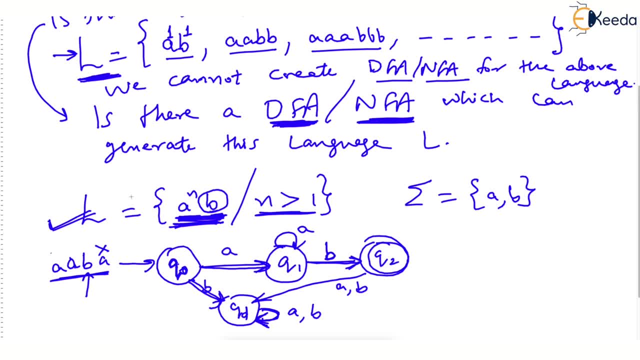 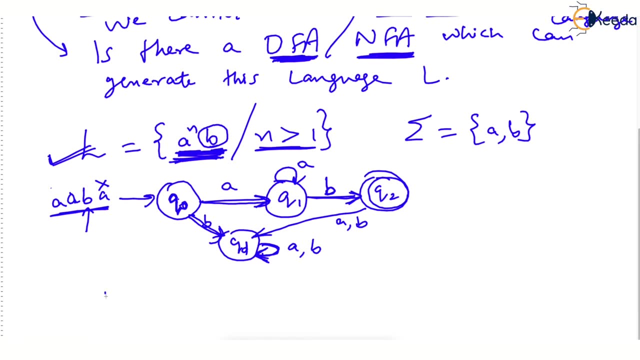 So is this language regular? Yes, it is regular because we can construct a DFA, Isn't it so? So what happens really is that given a completely a new problem on one fine day, you have been given a new problem as follows: 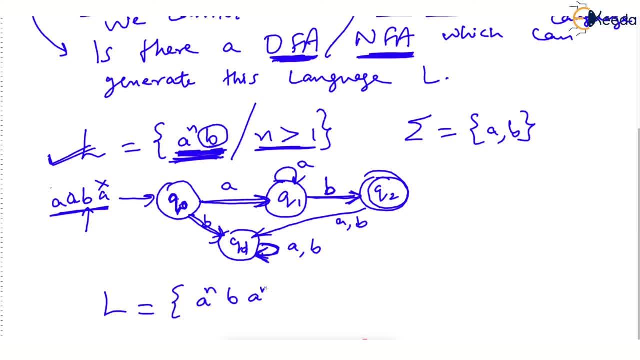 Take this language as a raised to n, b raised to n, a raised to n such that n is greater than 1, and sigma is a comma b. You are asked: is this language regular? Is this language regular? That's the question. 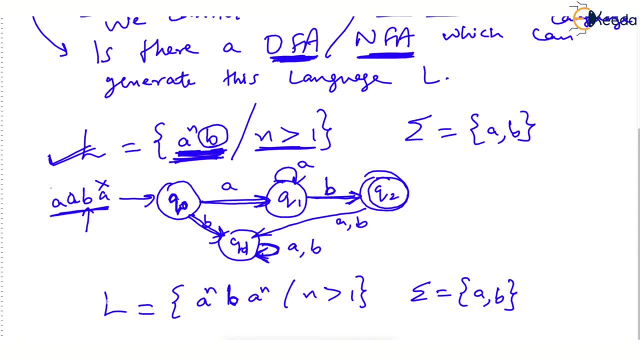 So what you would do? you would start very hard. you will start constructing a DFA And day, night long, you will try constructing, Constructing DFA, and then you will give it up. You will say no DFA. at least I am not able to construct a DFA for this. 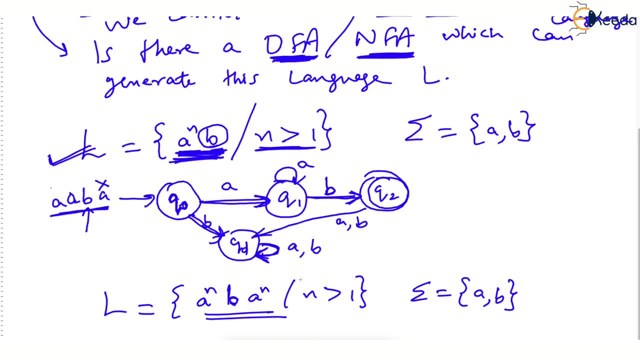 But then can you claim that this is impossible? Can you claim, and can you really raise your hand and say, that this language is not regular? Oh, you are in doubt. you are in doubt. You say: I am not able to construct DFA. 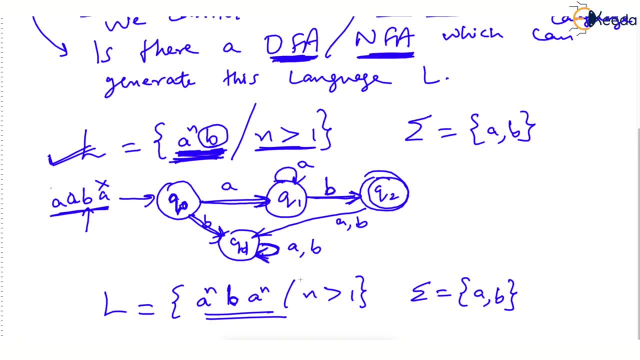 But, who knows, there might be an answer for this. So don't you feel that we need a solid proof When we are claiming, when we are claiming that this is not regular? this is not regular? we should be sure, isn't it 100% sure, that, yes, DFA is impossible for this? 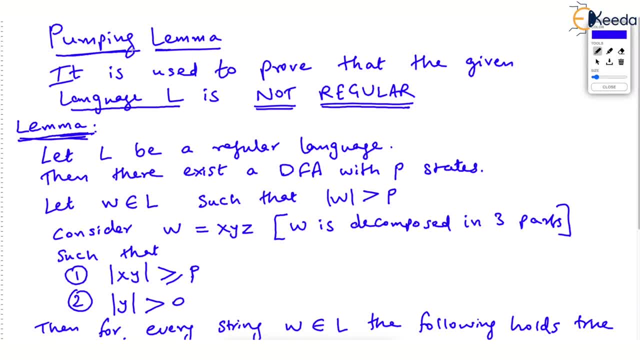 But then how do you prove it? Here comes the lemma pumping lemma. it is used for just check. it is used to prove that the given language, L, is not regular. You can use this theorem and you can straight away say that the given problem cannot be solved. 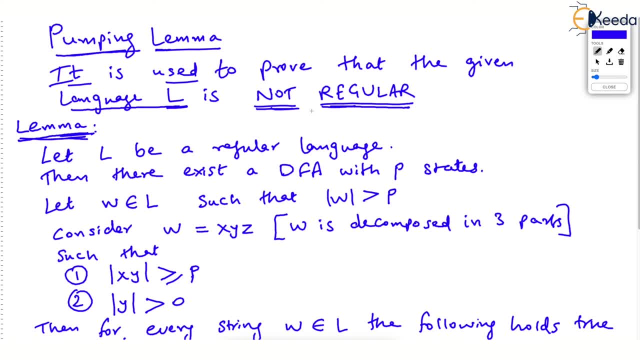 using DFA, by using the steps of the theorem. I hope I have made the things very clear. What is pumping lemma all about? And, trust me, once we know this, once we know this technique, you know. then assume that the language given L is something like this: